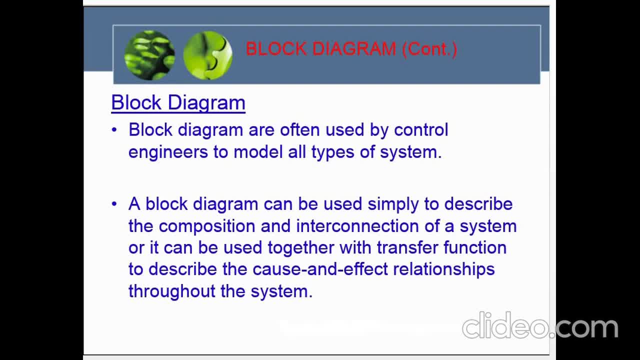 correlation with other. okay, a block diagram can be used, simplified, to describe decomposition and interconnection of a system, to create JUST a block diagram possible in computer language. or it can be used together with transfer function to describe the cause and effect relationship throughout the system. it is why the engineer use control system. 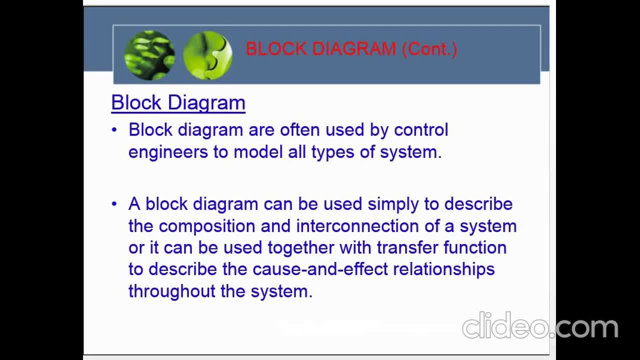 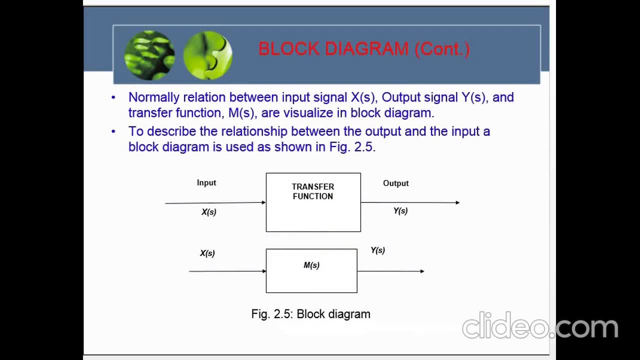 let me just block the agreement, sorry. okay, normally relation between input signal xs and output signal ys and transfer function ms are visualized in a block diagram as a figure. 2.5 is the block diagram where this input input is xs and there is the transfer function, it is the output ys or 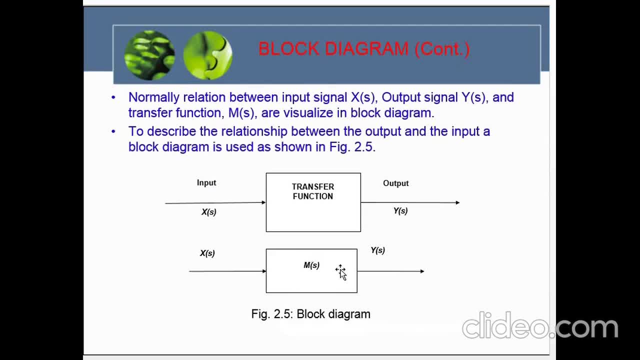 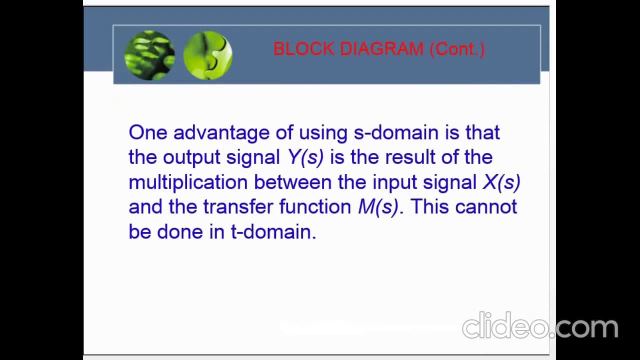 uh, we can write it in the block. in this block it is ms. ms, it is the transfer function. okay, one advantage of using s domain is that the output signal ys is the result of the multiplication between the input signal xs and the transfer function ms. this cannot be done in time domain. 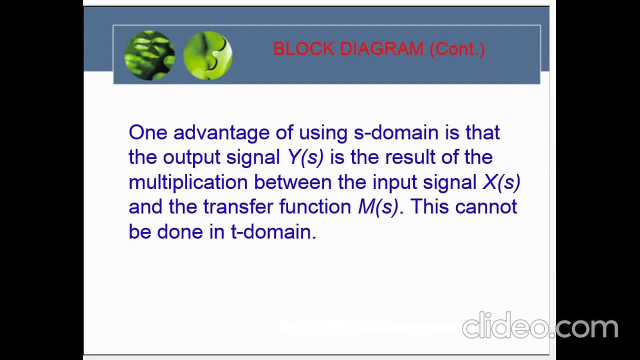 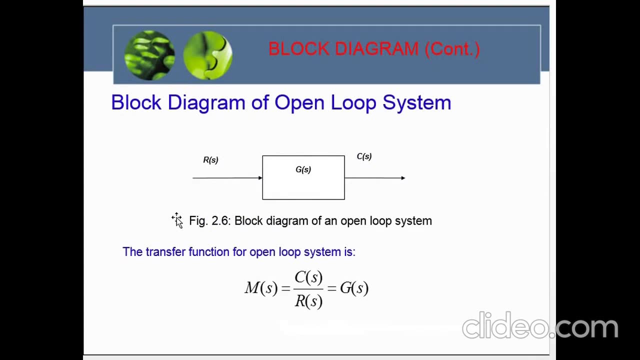 this is why in this subject we use laplace laplace transform. okay. block diagram of open loop system. this is the figure 2.6, so the block diagram of open loop system. you see, there is a rsdc input, gsd is the transfer function, csdc output. 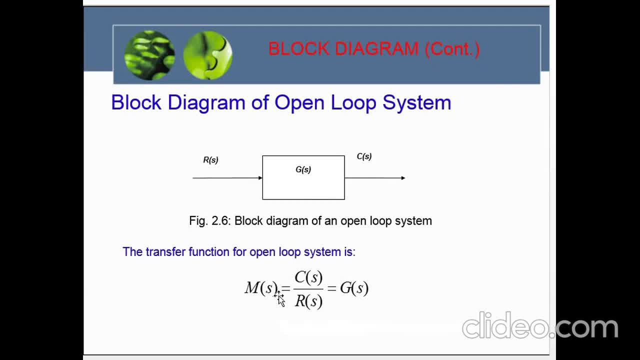 transfer function for open loop system based on this block diagram. it is ms, msu, equal to csprs, equal to gs. okay, this is a transmission for open loop system. okay, next we look at the closed loop system. gray figure: uh, two, seven, uh. so the block diagram of uh, a closed loop uh system. here we see, uh. 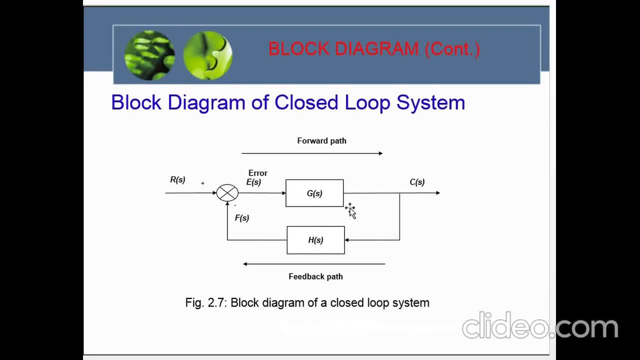 there is the feedback. that is the feedback, and there is the loop, uh, and there is the comparator, or uh summing point and the output. the input is rs and uh. this is the feedback signal. fs, the uh, rs, a minus, fs, this error, uh. there is the uh- forward gain or forward transfer function. 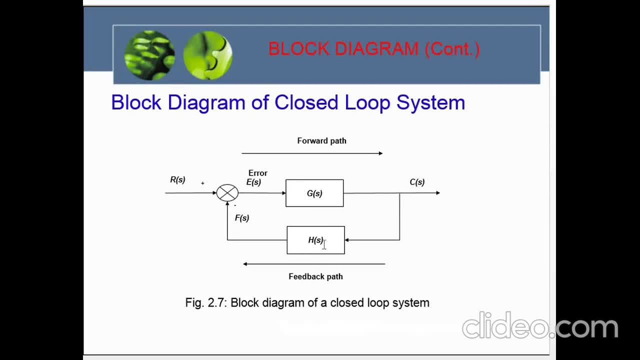 and there is the output headsets. this is the feedback gain, or feedback transfer function. feedback, uh yeah, the back gain, and this is, uh, this space we call the four- phrase and this space we call a comep quiere feedback phase. okay, uh, gs, this is a forward phase transfer function, or forward gain. 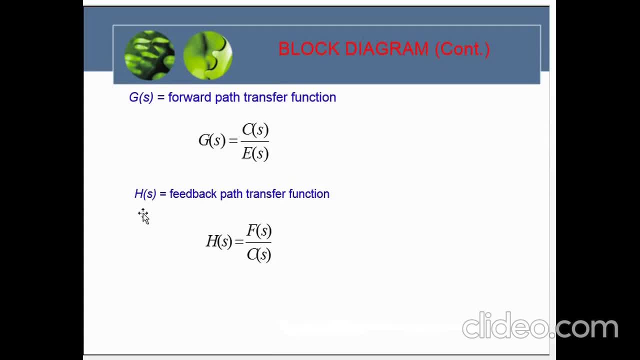 gs. this is cs per es and hss. this we call feedback phase, uh transformation or pd gain. okay, obtain the trans function of the system: ms the ms equal to cs per rs. that is equal to gs uh one per uh one uh uh the ms. this is equal to cs per rs. equal to uh gs per one plus gs hss. 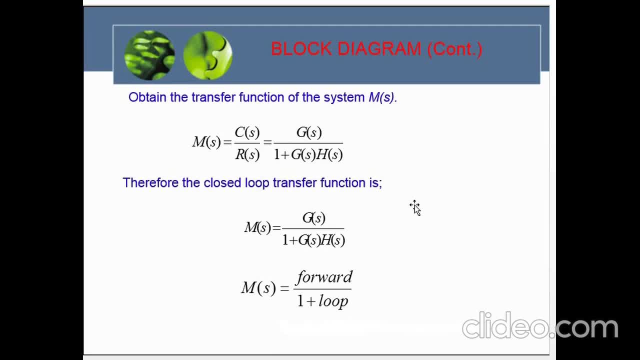 okay, uh. therefore, the closed loop transfer function is uh as uh below. this is the general formula: the ms equal to gs, uh per one plus gs, hss or uh forward, or forward gain, our power transfer function. divide it with one plus loop, uh, loop gain. okay, this is the general uh formula. 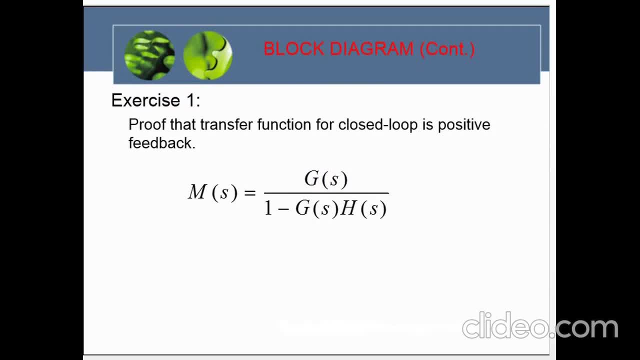 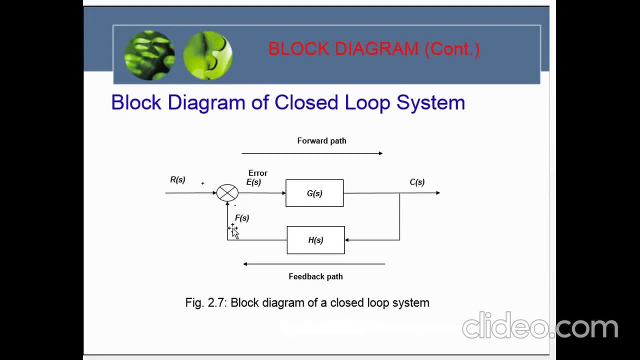 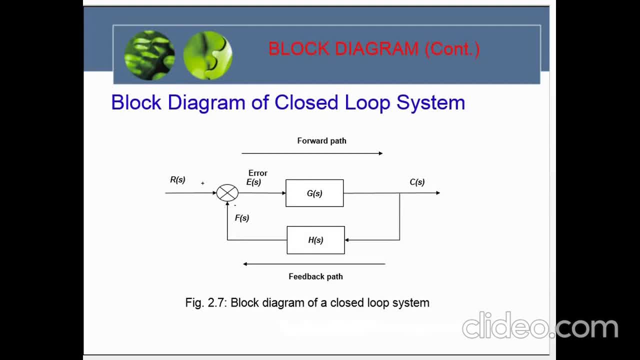 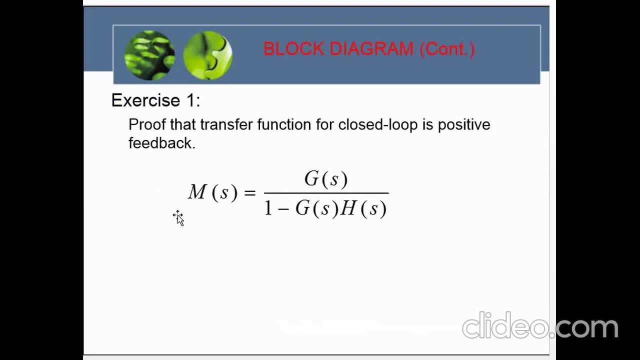 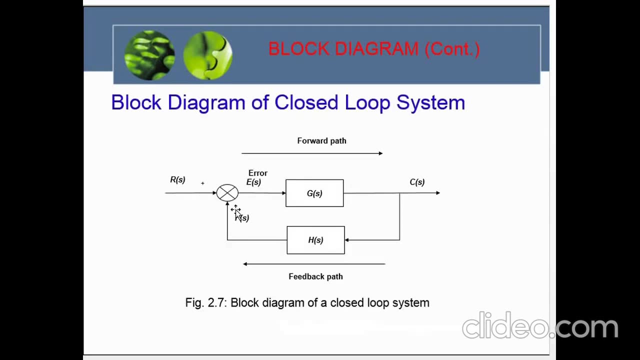 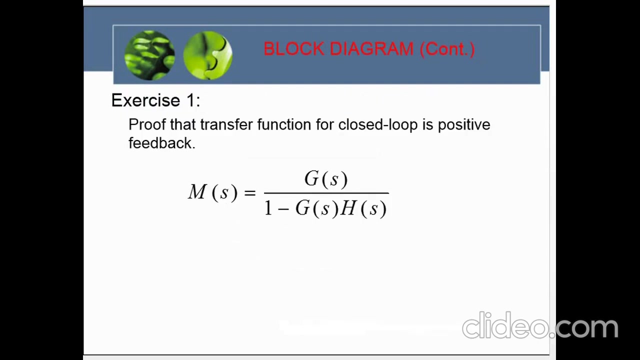 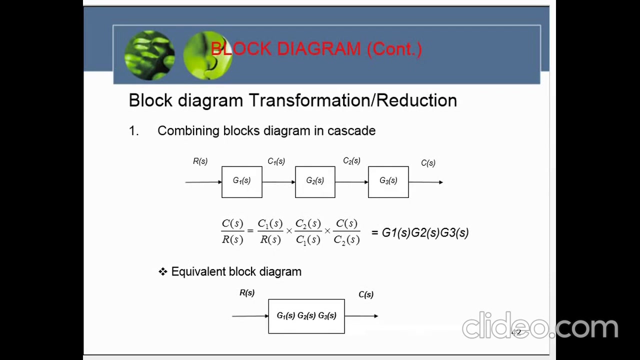 of this time it is negative, okay, but here positive feedback, positive feedback. and then you asked to be rapid. it means a change, design become plus and please prove this formula, okay, okay. next we look at transformation or solution combining. you see, here there are consists of three blue bedroom, with gain, it is. 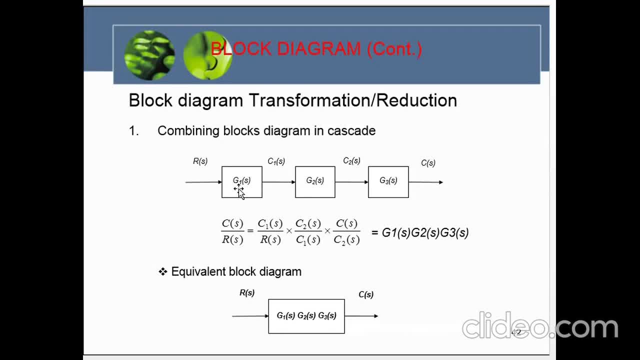 already run. reden القаемous trans function. g1s, g2, g3. okay, there is the input for g1, rs, the output is c1 and then c1. this become the input g2 and then the output g2 is c2 and become the input for g3 and the output of g3. 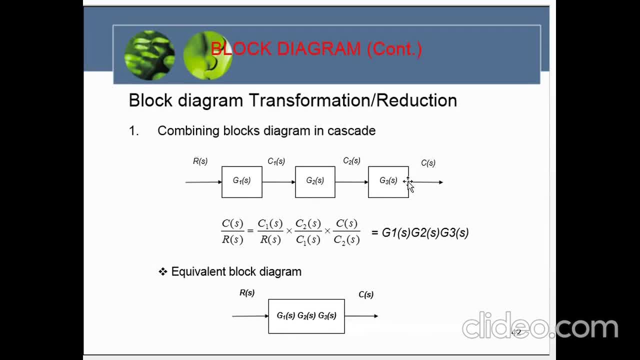 is cs, and also the output, that the total output, the total output from this system, okay, uh, cs per rs, is it mean uh transfer function for all this equal to c1 per rs, c, the multiple c2 per c1, multiple c per cs is a c2. i'm sorry. and then we know: this part, it is g1, and this part it is g2, and this: 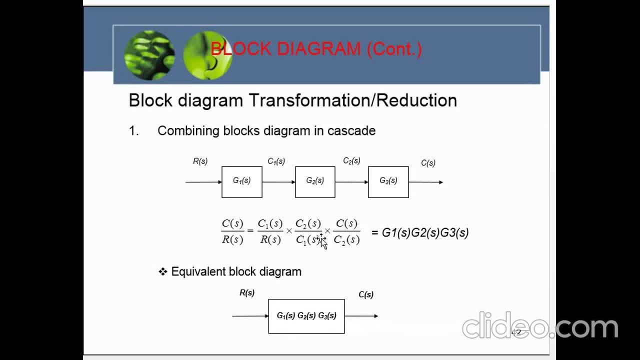 well, this uh, this part, is g3, and then we change this. it is become like this: rs per uh, cs per rs equal to g1s multiple g2s, multiple g3s and equivalent block diagram for this block release. this is the simple uh block diagram. okay, this simple block diagram. we reduce this, become simple like this: 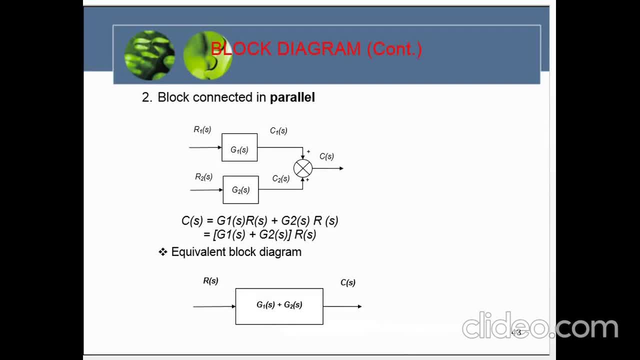 okay, number two. uh, block the block connected in parallel. okay, if you see, here it's the block diagram. uh, this, uh summing point. first block: uh, the input it is r1 s, transformation is g1s. the output is c1s. okay, and uh, it is the number two, this r2s. 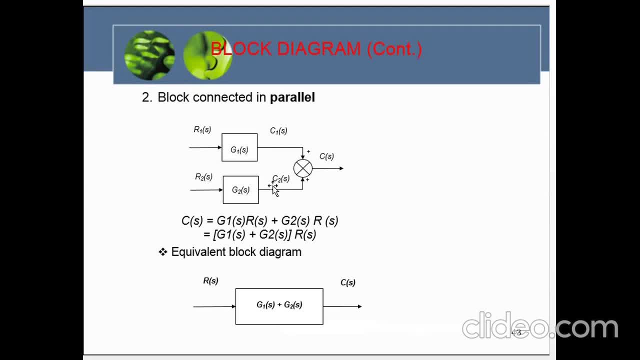 g2, uh, s, and then the output is u, uh, 2s, the total output is cs. if uh, in this case we assume that r1 is equal to r2s, equal to rs, okay, we see here: uh, uh, cs. cs is equal to uh, g1, cs. cs is equal to c1s plus c2s, or equal to c1s is equal to g1. 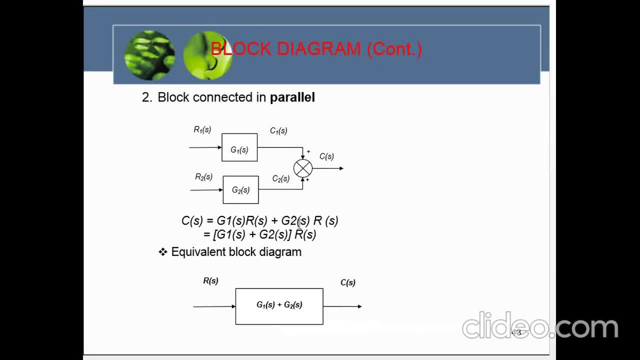 rs and then c2. this is g2, rs and then uh. at the end we simplify and get that: uh cs. it is in the bracket g1s plus g2s. uh, close bracket it is rs and this is the uh. simple block diagram. simple block diagram. 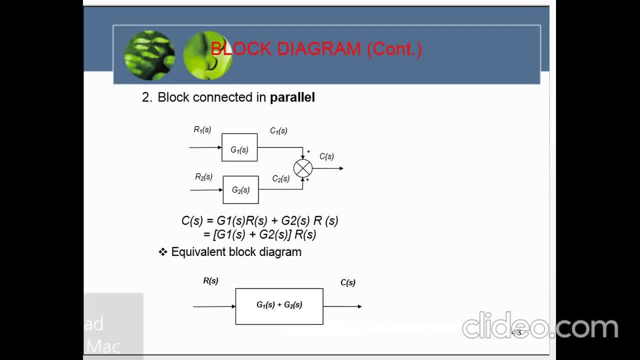 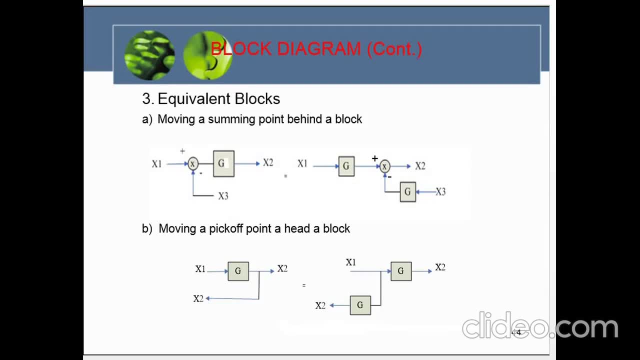 okay, okay, uh, equivalent block diagram. okay, uh, this, uh uh, separate principle: that, uh, you want to study here, uh, in this, uh part first, it is a moving, a summing point behind a block. it is the summing point. we move it after g, uh, okay, the result. the result must be the same, okay, first. 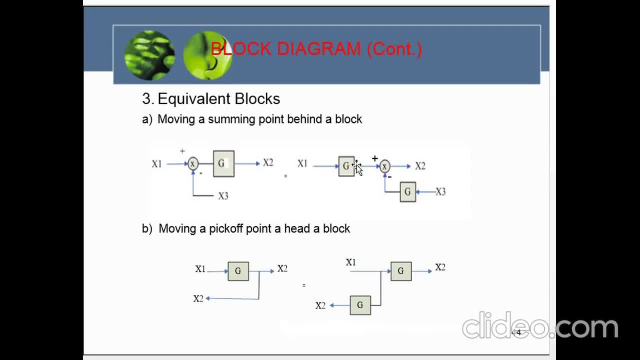 we move it after we move the summing point after G. okay, we look at here the output. it is G 2 is X 2. I'm sorry, X 2 X 2 is equal to X 1 G minus X 3 G. okay this. 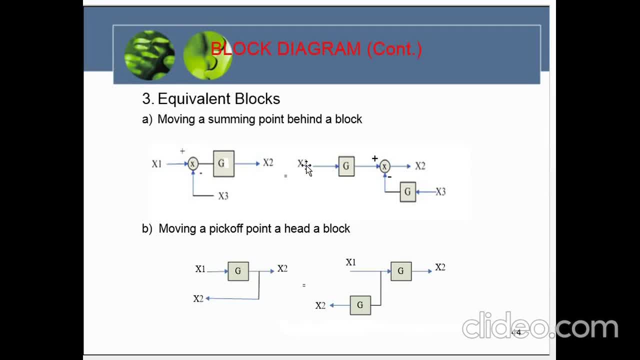 is the output we see here. X 2, it is equal to X 1 G minus X 3 G. this is the same, it is true. need. how to verify our work? it is true or wrong? okay, next, moving a fixed point ahead of a block. it is the summing point. it is the fixed. 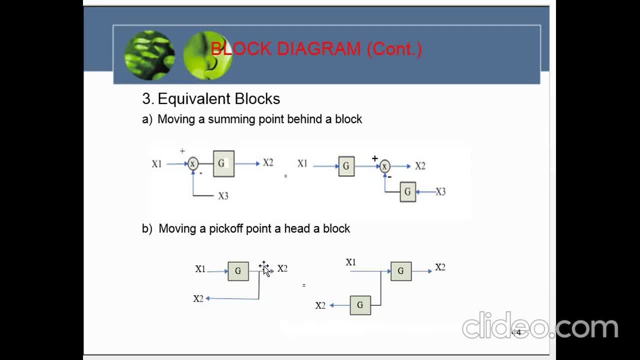 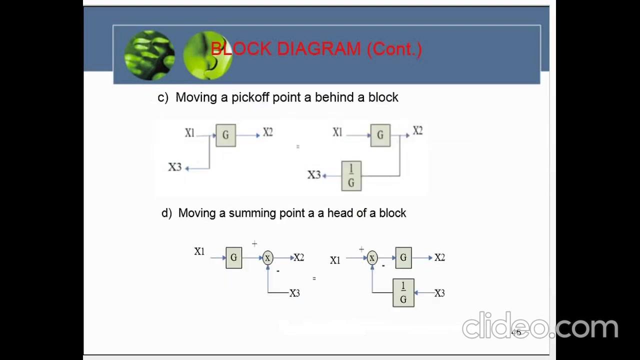 point. we move this point before the block. that is the that we get. we see here: X 2, it is equal to X 1 multiple G, and this output also X 1 multiple G, and it is after we move. we see the result: x2, it is equal to x1g and here also x1g. yeah, it means our work. it is okay, okay. next. 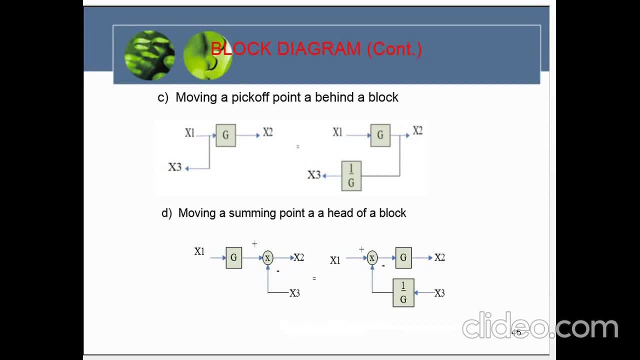 moving a pixel point behind a block, it is the fixed point. we move it after g if first we determine the output. here output 1, it is x2, x2 equal to x1g. x3 it is equal to x1. after we move it we check again the same or not. here x2 it is x1 multiple g. and then, because of here, if we move, 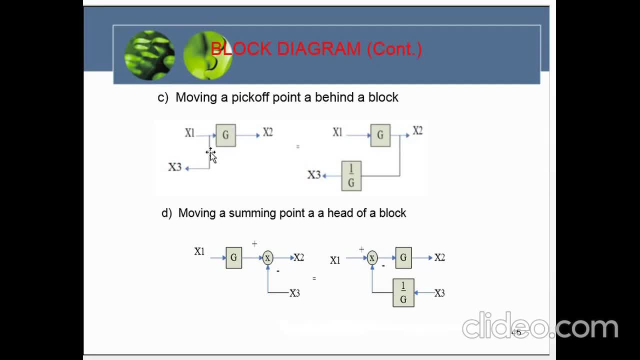 here g, it is include in x3. how to eliminate it? we give gain one per g, g per g, multiple one per g, this become one. okay, we get again x3. it is equal to x1 and this true. this is the mechanism. the last principle is moving a summing. 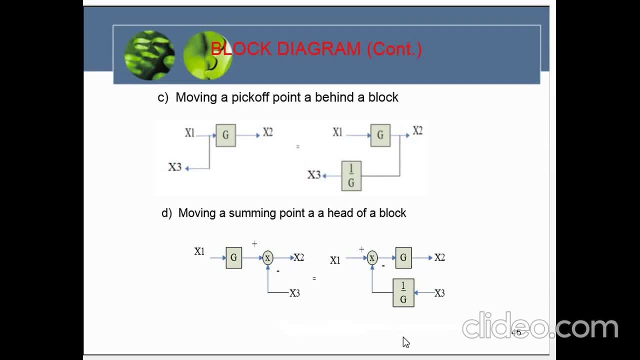 point ahead of a block summing point. he move ahead. for example, this: we move this summing point before g, but we first we checks the output. the output of this block, it is x2. here we see that x2 equal to x1g minus x3. and then, after we move it, 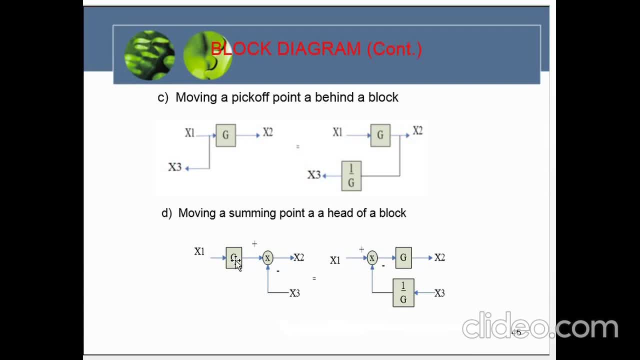 x2 change because our work this k as k1 we are going to reduce immediately because it is little. we are saying that k is one, in c2 it is 101, j6. here we go. we know that xn equal to x1, actually g because of kaze value, because 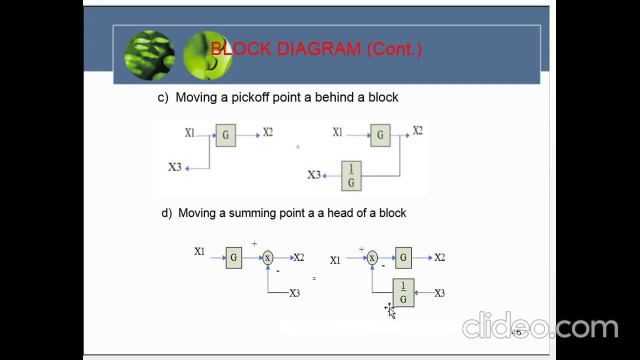 each g here in g, what is k b zero? this k a e, a b which we got from? if this not, are the gain Hotel checked and it provided a 5. distillation. similar situation, rather similar situation, usually a sinus, but here we move t, here there is a 3. distillation. 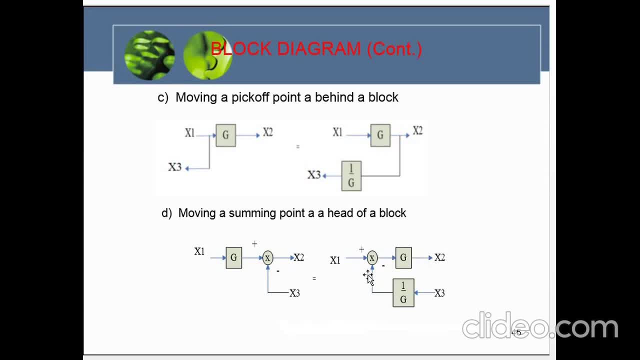 g, also what this 3 being known as kj. we multiply the rate, this is the distance from, by g and x2 is the here x1, here in this condition, x1 plus minus x3 per g, and then if we multiple g, and then we get that x2 equal to x1, g and minus x3, this still the same. okay, this it mean what? 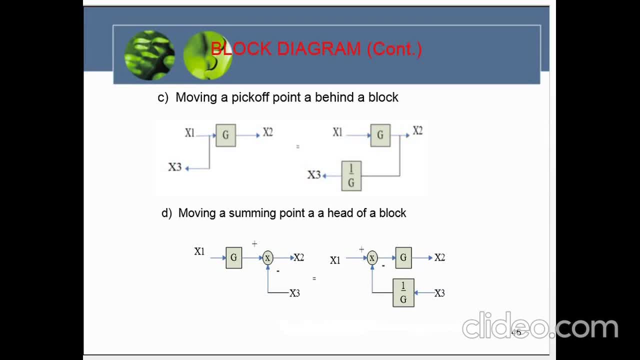 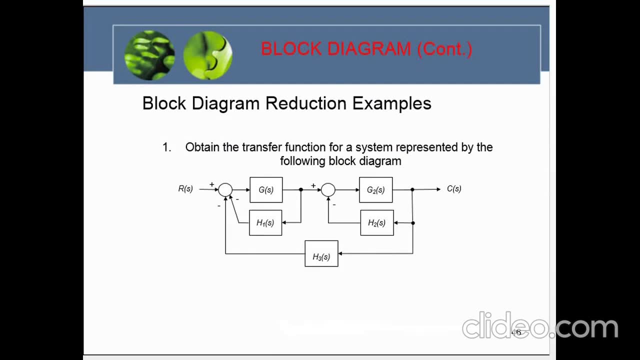 we have done, it is true. okay, now we try to apply it. we try to apply the concept that we have studied previous. okay, this is the example. we ask here to reduce the block degree and in order to get the simple one, okay, if we see here the block. 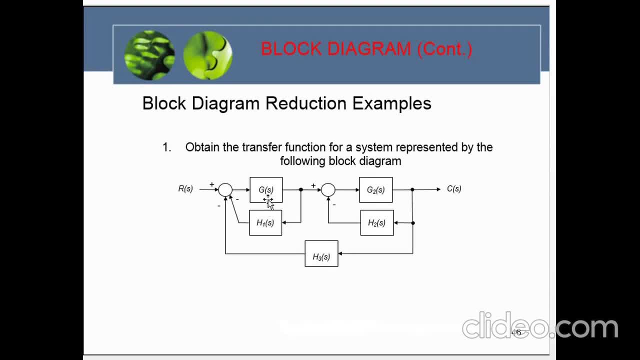 theorem is consist of three loop. it is the first loop and there is the second loop and there is the third loop, but this loop not independent and this loop was not independent. it is difficult to about to simplify it. in order to simplify this, we must separate this summing point. okay, although this at the fixed point, we should move it. 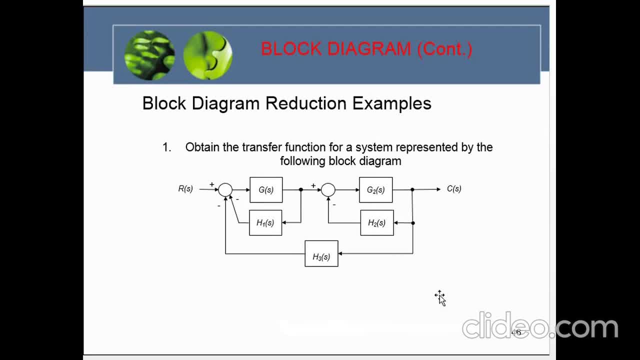 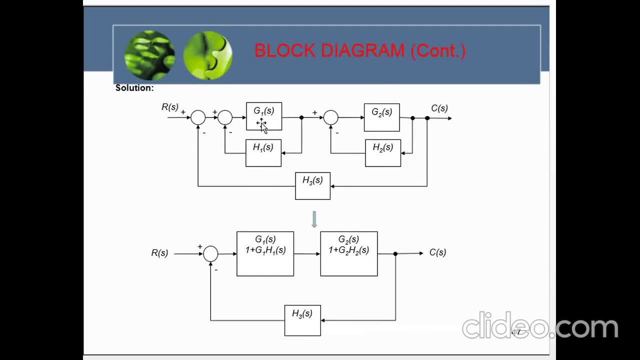 in here and it also we move it here, okay, and we get like this: okay, it is free, it is free, okay, by using the principle of today, general form of the transfer function formula, and then we get this and the transmission of this, but this and transmission of this part areas, okay, now 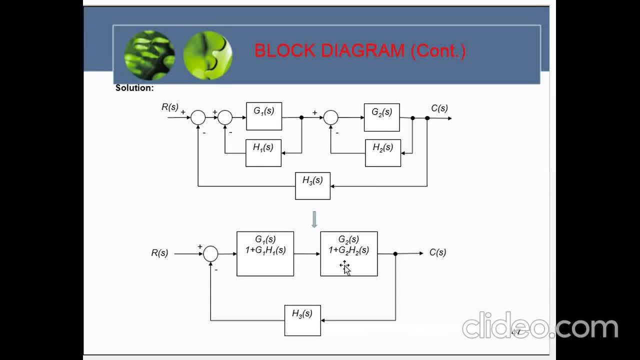 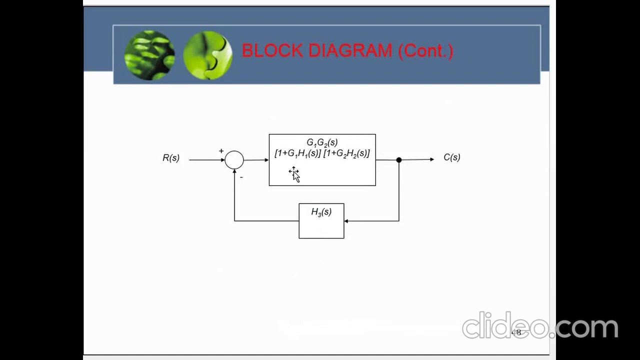 we get the block diagram like this: okay, this is a cascade and if difficult to you direct to determine the this transfer functions for the this loop, the last loop, you can cascade it first. okay, this is the cascade of two purposes and it is a cascade g1, g2, third in the bracket one. 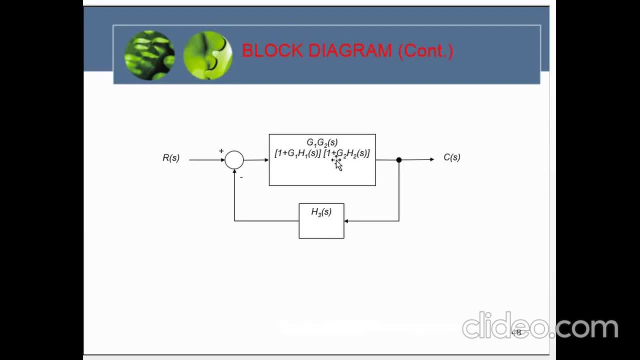 plus g1 has one close bracket, multiple open bracket. one plus g2 has two close bracket and there is the it feedback. okay, because of this, the negative feedback. we know that negative for negative feedback. it transmission: it is forward gain per one plus loop gain. okay, it is the formula. and then we get it and 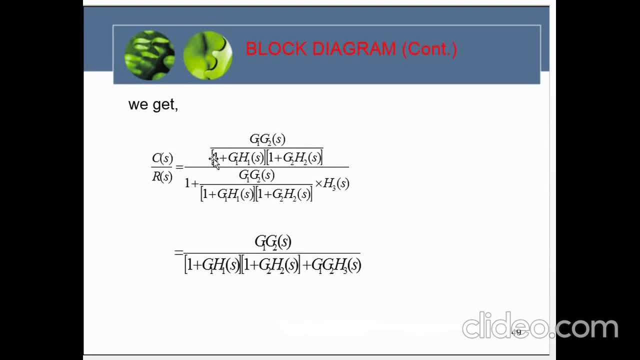 it is. if we substitute, it is for forward gain, it is one plus, it is forward again, multiple feedback gain. and there is that last week it is: this is the transfer function okay. and if we make the simple or we draw the simple box you can see here, it is like this: okay, it is the transfer function okay. and if we 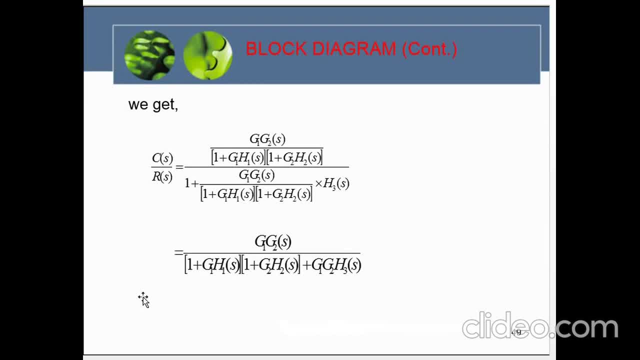 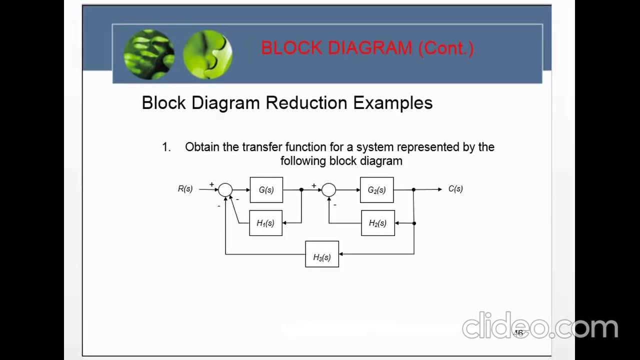 make the simple, or we draw the simple box and then here here the input rs and then in the block diagram you can take it and the output is cs. okay, now, if we apply the uh, the concept that we have studied for this, how uh for uh, reduce. 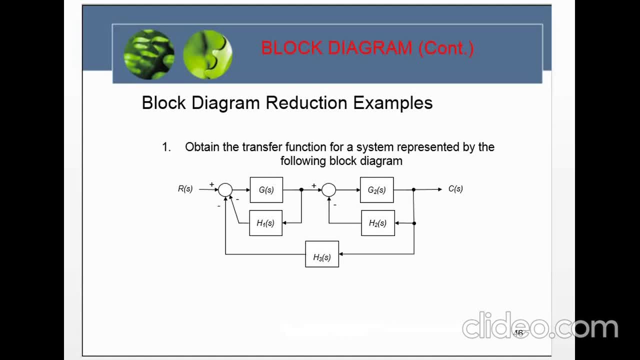 the block diagram- it is the example of local diagram- consists of three loop and it is first loop, second loop and, uh, there is the third loop. that is the feedback for uh, loop one and then loop two and loop three and then now the first step, uh, to mix each of the loop independently. okay, 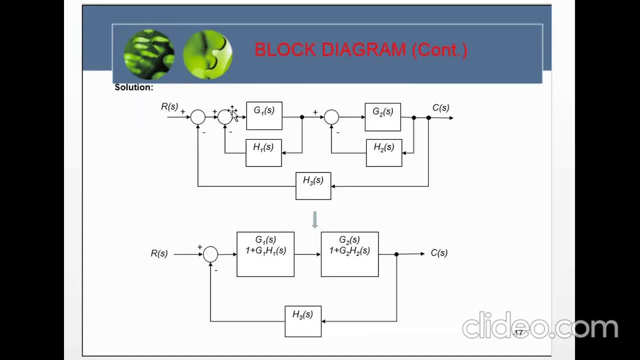 okay, this, we uh separate this feedback into this summing point and by uh at a one uh summing point. here again: okay, this loop uh free and then also this point from here, purposefully uh move it here. okay, and although this loop become free, okay, now we can uh determine this uh loop transfer function. 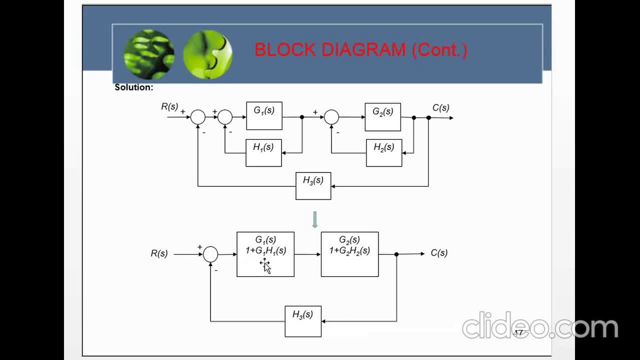 this is the transfer function and how to uh uh determine the transfer function. i have uh, so you practice. and then there is the transfer for uh uh, second loop, and the result. this result, it is the casket, casket, uh. and then uh, we uh simplified it first before we uh simplify the last uh loop. 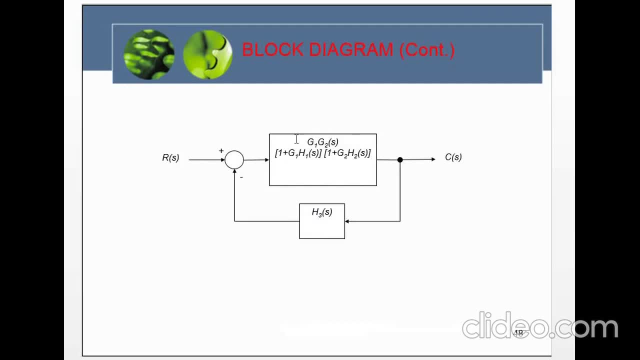 okay, and it is uh the simplification of the casket, uh, uh gain or the cascade block. it is the uh, it uh simplified the g1 uh, g2 uh divided to uh. in the bracket, one plus g1 has one uh close bracket. in open bracket, this one plus g2 has two close brackets. 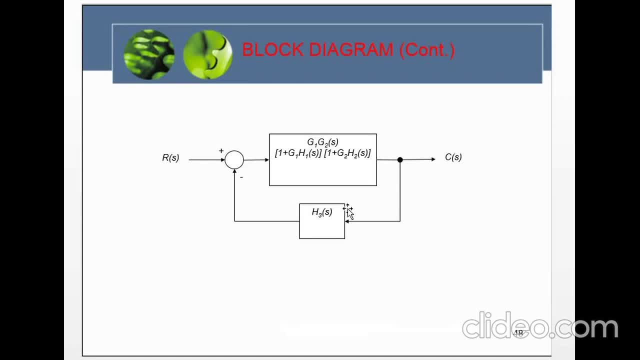 okay, and it is the uh feedback of uh third loop. okay, now this uh have been simple and we can use the previous uh transfer function formula. yeah, general formula that i have u" uh, so you get transformation equal to forward again per uh one plus uh loop again, or? 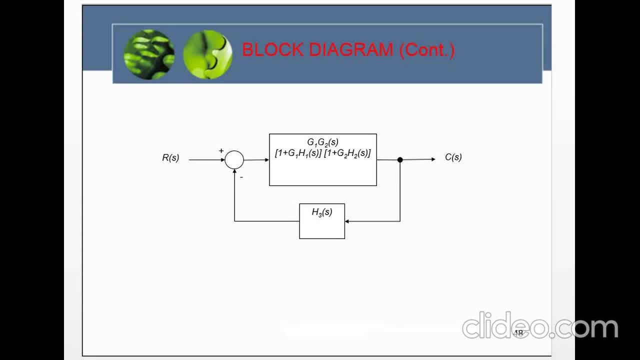 g uh s for one plus b s s s. okay now, uh, by using that general formula, we getデ, But we get d's S ed to"s a mine the last. this is the simple transfer function, or the simple model, and this is you. we can take it. 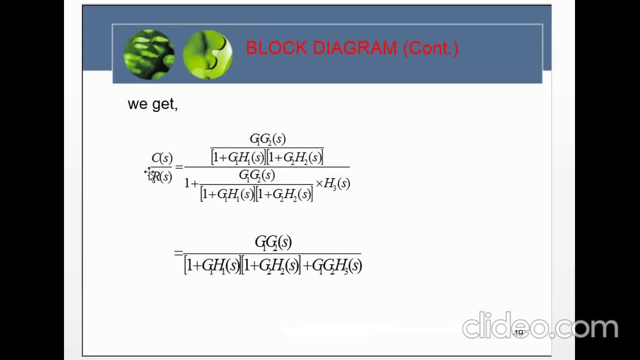 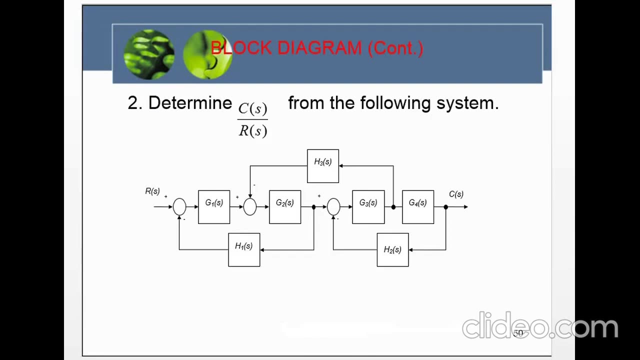 into the block and this is the input, rs, and the output is cs. if we, it is the final block diagram. okay, the first uh example. next we look at the second example uh determine the cs for rs uh from the following uh block diagram: block diagram: this block diagram: it is uh more complicated. 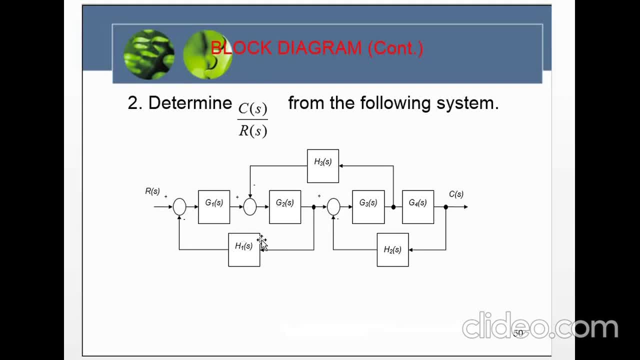 than previous. it is also conceived- consists of: uh, three loop. yeah, this is first loop, second loop and the third loop and now, uh, in order to make free, in order, we should move this point, this summing point, uh, this, uh, this point before g1 and then this is before, after g4. okay, it is the mechanism and then, if we move it here, 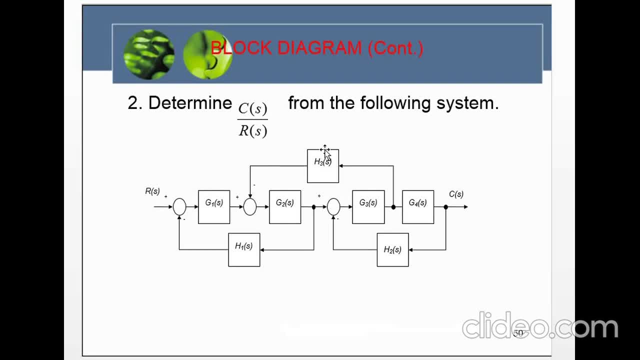 we move it here in order, the result is still the same. if we see, if we move it here, it is the feedback here: G1. it is not content here. error G4. although not content in here. this loop and how to eliminate it. it is by doing: